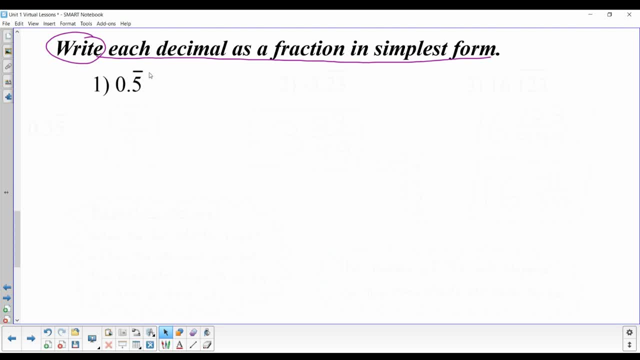 Hello, in this video we are going to go over turning decimal, repeating decimals, into fractions in simplest form. Please be aware, the method we are going to show is more of a shortcut and only works if the bar notation or the bar is immediately over the first digit after the decimal point. 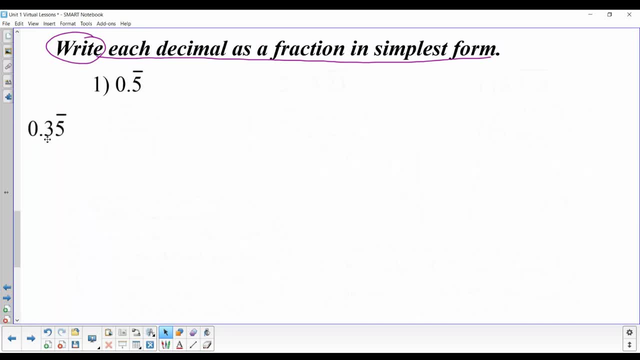 If you have a problem like this example here- 0.35 repeating- where the bar does not start immediately after decimal- then what I'm showing you is not going to work and you have to know a more advanced method, which we'll go over in a future video. So, if the bar starts immediately, 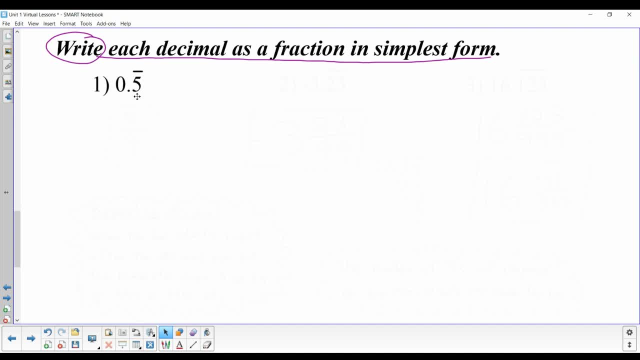 after decimal point. all you have to do is take the number after the decimal, and this is number one, five, and put it over a nine and that's it. If you have one digit that is repeating, it goes over a nine. Now, if you have a problem like number two negative 3.23, repeating where there are two digits, 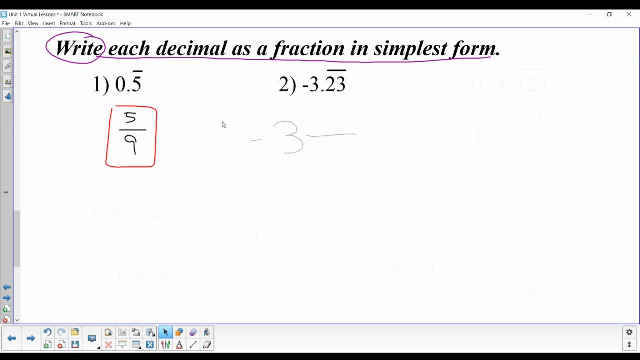 repeating any integer or whole number you have stays an integer or whole number. negative three stays negative three And the decimal part becomes a fraction. Whatever is after the decimal, in this case 23, goes in the numerator and since there are two numbers repeating, you would put two nines in the denominator and 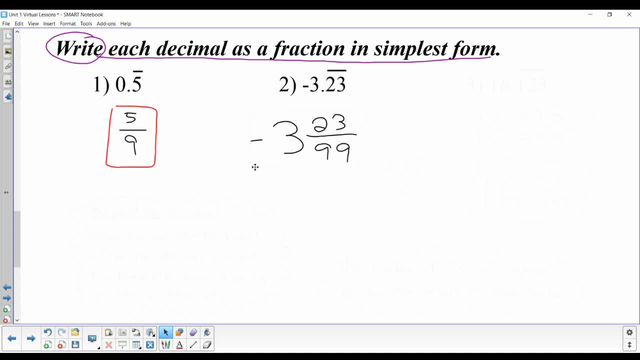 since there is no number that goes into both 23 and 99 besides one, we cannot reduce this fraction. I'm going to do a third example. problem number three and what I want you to keep in mind are two things. One, when the bar starts right after the decimal point, the bar starts immediately after. 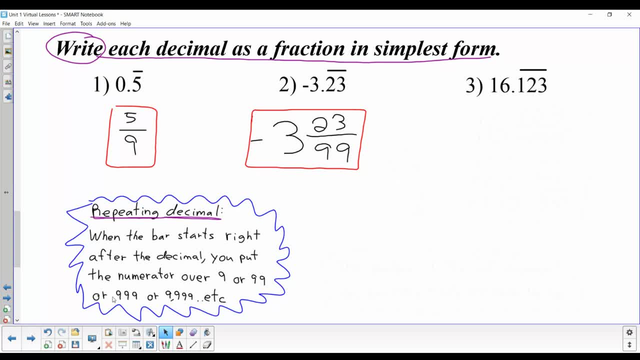 the decimal point you put the number over a nine or a 99, or a 999 or a 9999. it is always over nines and to know how many nines you have to have it over, the number of nines will depend on how many. 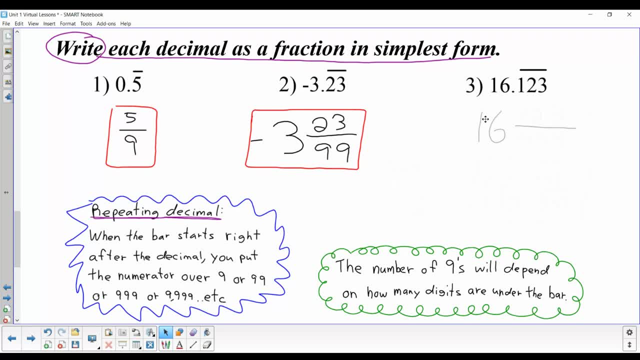 digits were under the bar. So, for example, number three, we have 16 and it's going to be a fraction, since the number after the decimal thing, 123, 123, goes in the numerator and since there are three numbers after the decimal Poin, There are some numbers a little less than the decimal one. and you can say that there is just three figures that are left after the decimal point, to have the one And, for example, number three, we have 16 and it's going to be a fraction, the number after the decimal 13, the number that is 123, 123, 123.